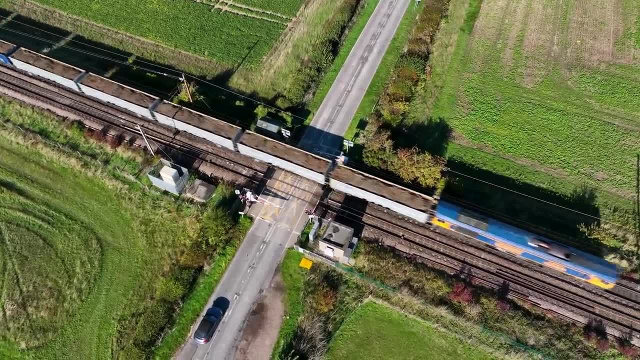 always have to be in a safe place. If you're in a safe place, you don't have to be in a safe place, You have the right-of-way. when they cross a road or highway at the same level or at grade, The cars 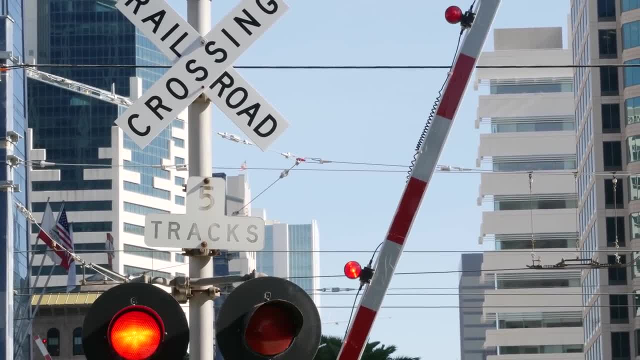 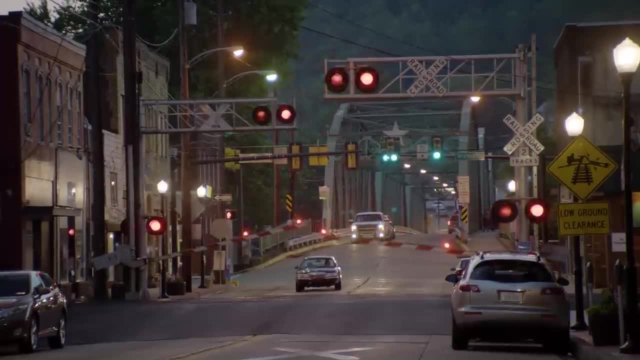 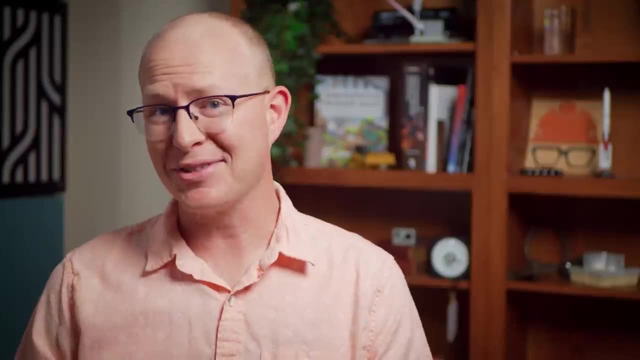 have to wait and we use a litany of warning devices at grade crossings to enforce that right-of-way and try to prevent collisions. In most cases, these devices have to detect the impending arrival of a train and give motorists enough time to clear the tracks or come to a stop. It sounds simple, but the 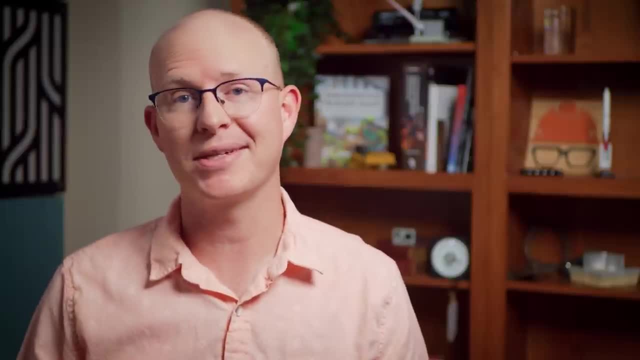 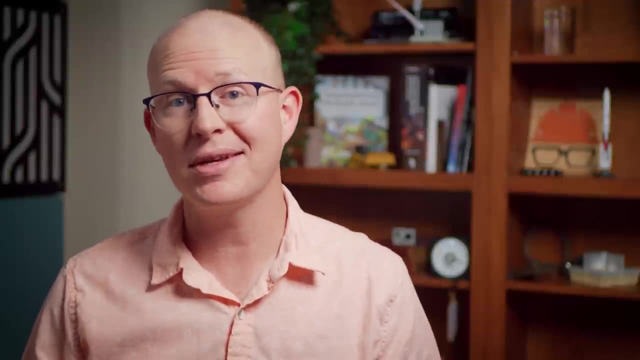 engineering that makes this possible is, I think, really interesting, And, of course, I built some demonstrations to help explain. This video is part of my series on railroads, so check out the rest after this if you want to learn more. I'm Grady and this is Practical Engineering. Today, we're exploring how 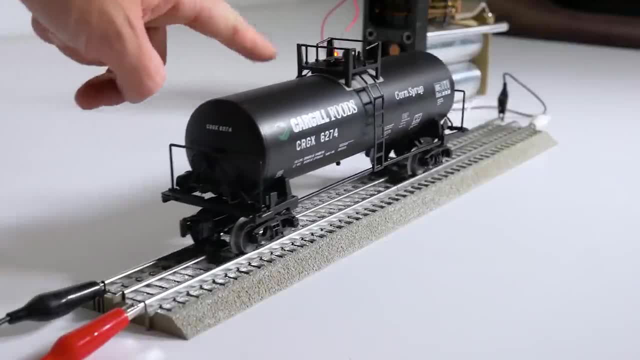 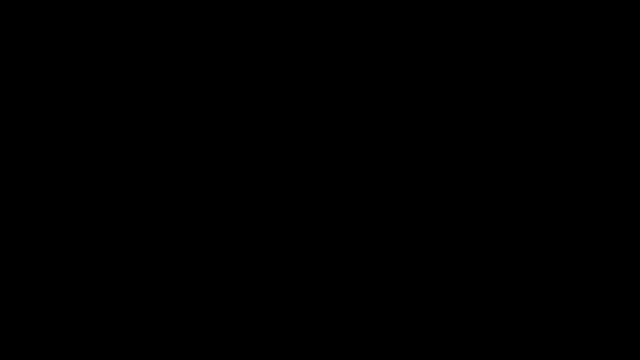 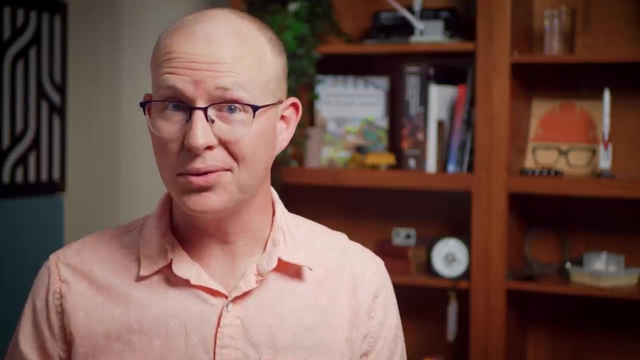 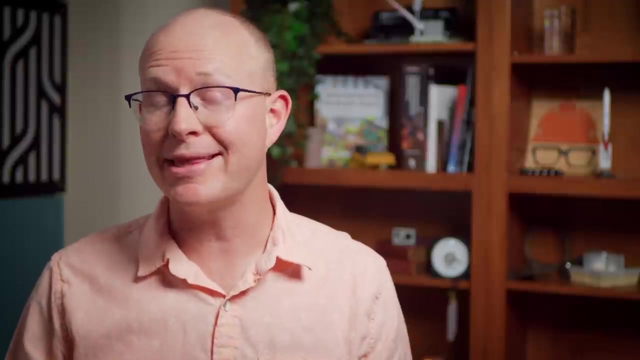 great crossings work. It's inevitable that roads cross railroad tracks and it's just not feasible to build a bridge in every case. In the US alone, there are over 200,000 grade crossings where cars and trains have to share the same space. A car to a freight train. 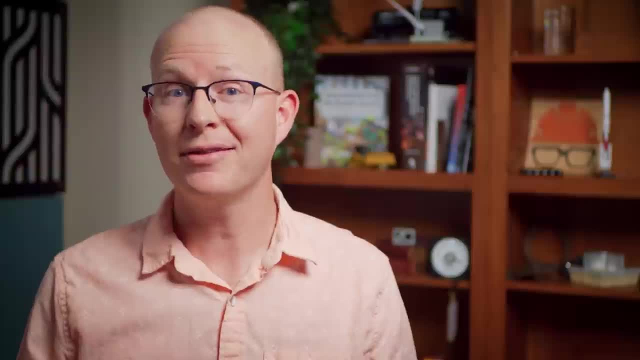 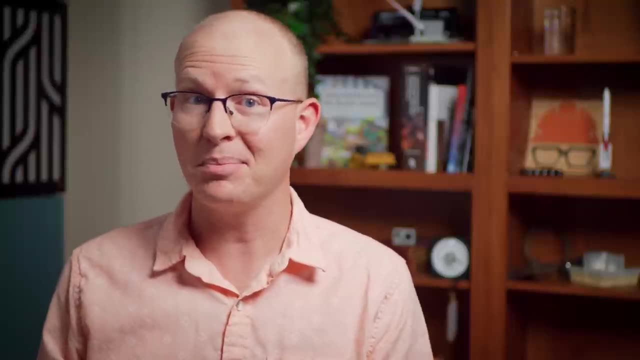 is an aluminum can to a car. In other words, there's a pretty big disparity in weight. so we've put a lot of thought into how to keep motorists, cyclists and pedestrians safe from trains that can't swerve or stop for a hazard. You've probably stopped for a train at a crossing, but 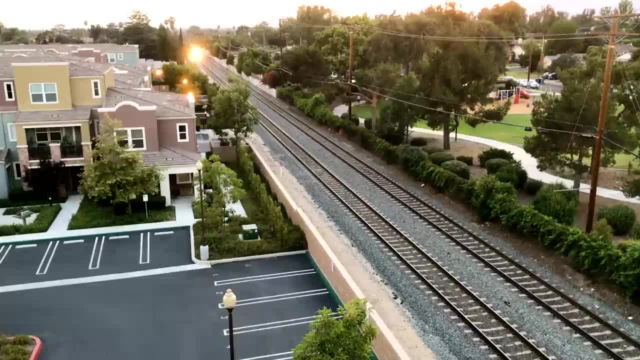 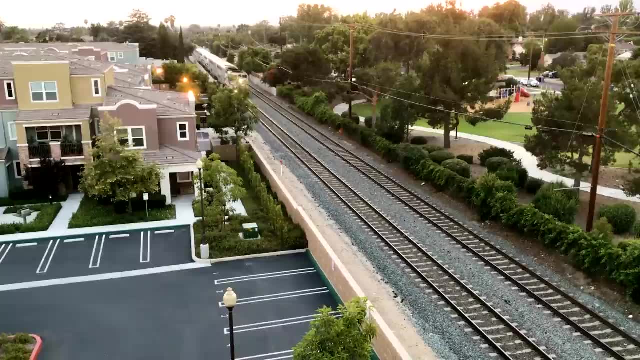 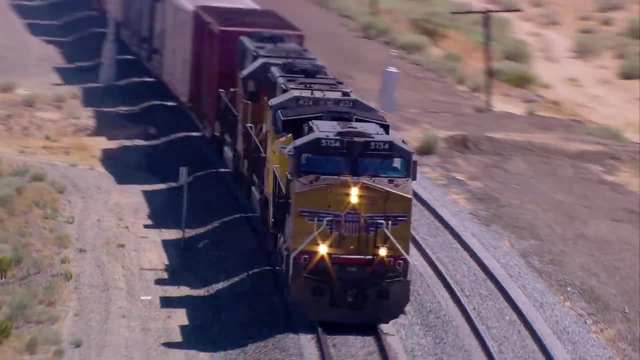 you may not have consciously added all the safety features up. Of course. the locomotives at the front of the trains themselves have warning devices, including bells, bright headlights, smaller flashing ditch lights and, most noticeably, the blaring horn. The standard pattern at a crossing is two long blasts, one short blast. 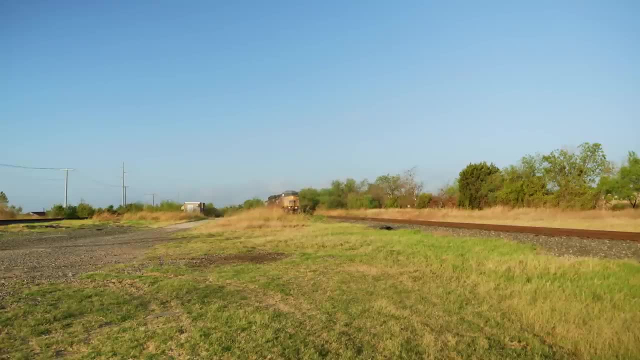 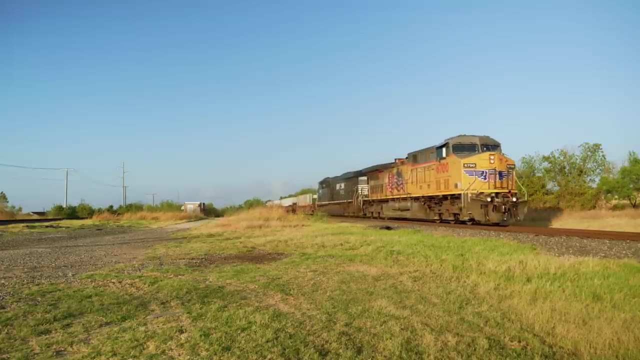 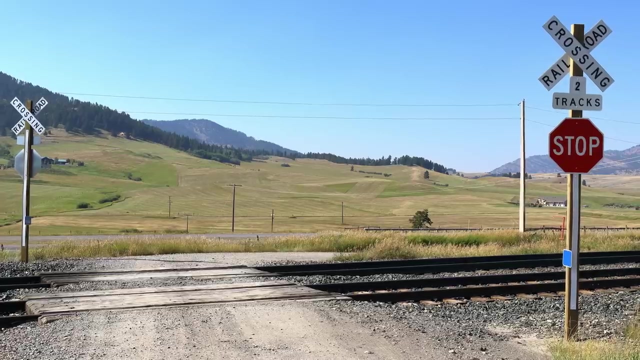 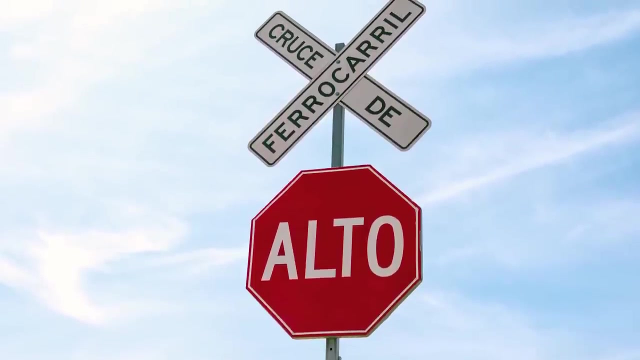 and one final long blast. But the crossing has warnings too. Passive warning devices don't change with an approaching train. They include stop or yield signs, the crossbuck, which is the international symbol for a railroad crossing, and sometimes a plate saying how many tracks there are, so you know whether to look. 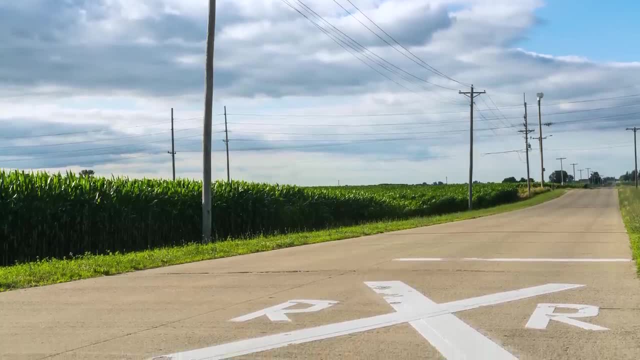 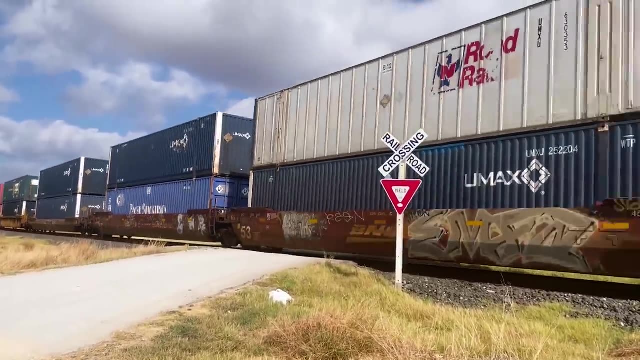 for one train or many. Another crossbuck is usually included as a pavement marking to make sure you know what's coming up. Many low traffic crossings have only passive safety features, leaving it up to the driver to look out for trains and proceed when it's needed. 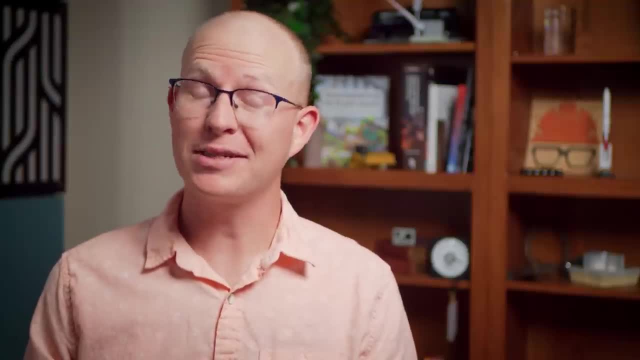 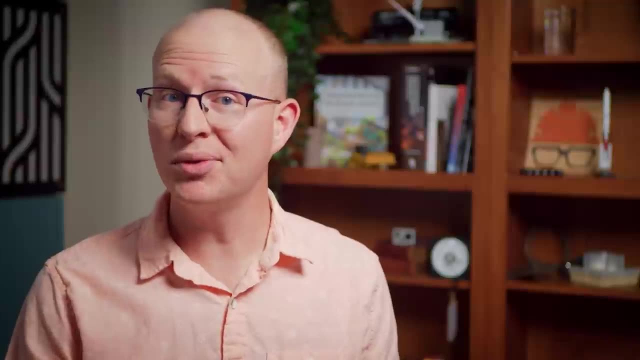 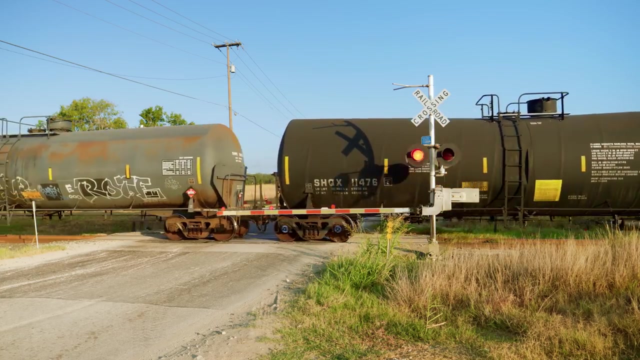 it's safe. But many crossings demand a little less margin for error. That's when active warning devices are installed. A typical grade crossing features both visual and audible warning signals that a train is coming. Red lights flash, a mechanical or electronic bell sounds, and usually 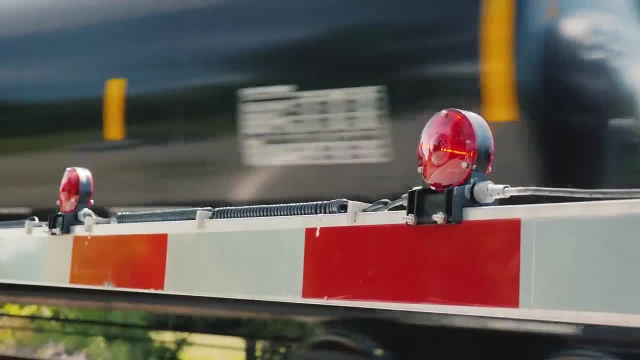 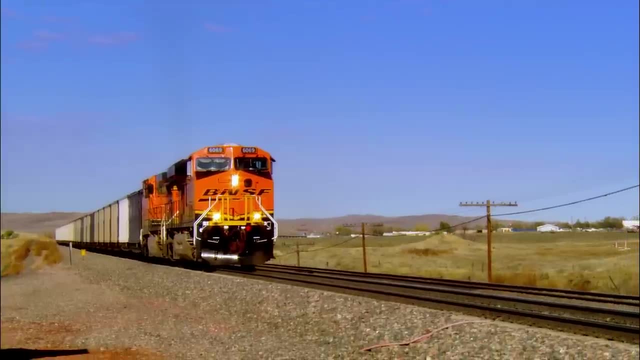 a gate drops across oncoming lanes. That seems pretty simple, but there's quite a bit of complexity in the task and the consequences if anything goes wrong are deadly, And the first part is just knowing if a train is coming. Detecting a train is important for grade signals. It's also important. 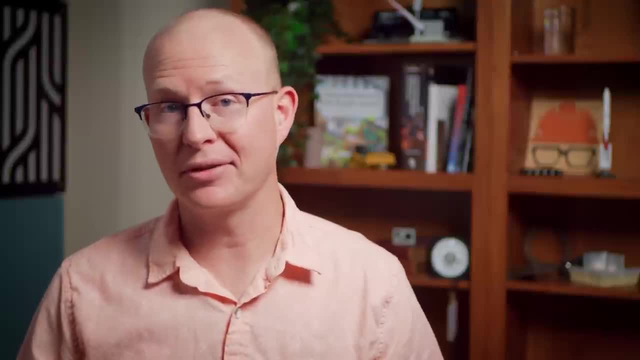 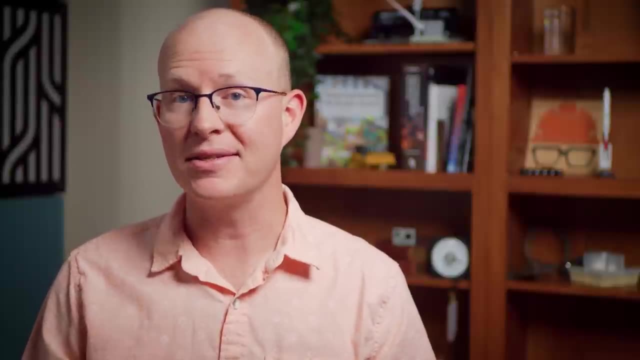 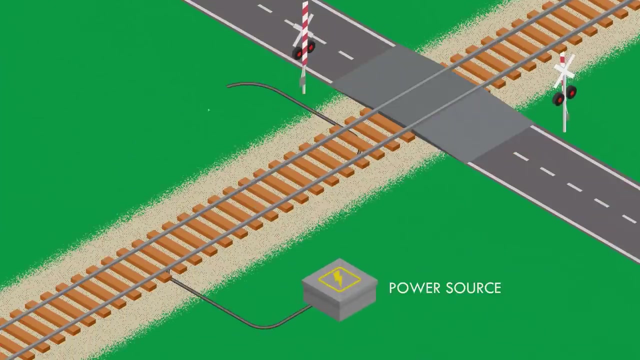 for signaling trains about other trains, but that's a topic for another video. It can be handled in a bunch of ways, but the simplest take advantage of the electrical conductivity of the steel rails and wheels themselves. A basic track circuit runs the current up one rail through a device called a. 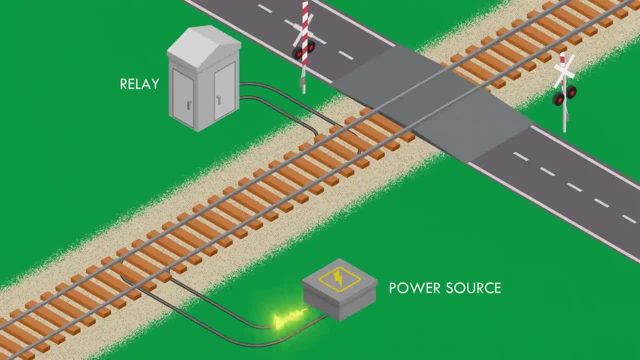 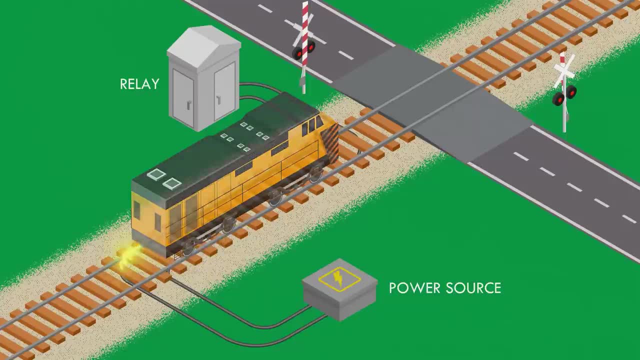 The train is running through the track at the end of the relay, generating a short circuit, a preferential path for the current in the track circuit. that de-energizes the relay, triggering all the connected warning devices or signals. But why use an ordinary old diagram when? 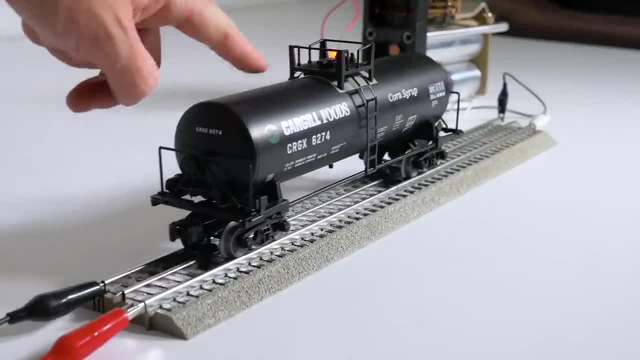 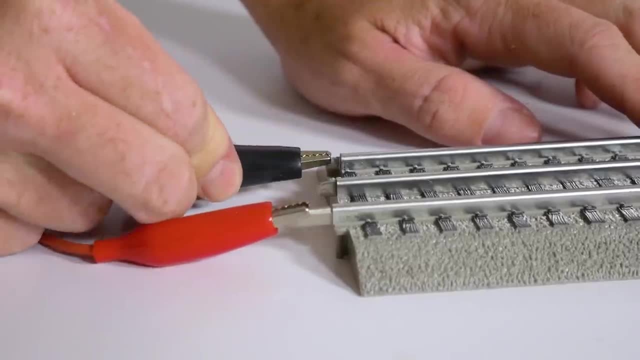 you have a model tank car and an old railroad relay you got off eBay. Let me show you how this works in a real demonstration. On the left I've hooked up a power supply to the tracks, putting a voltage between the two rails. On the right side, I've attached a relay. Let's take a. 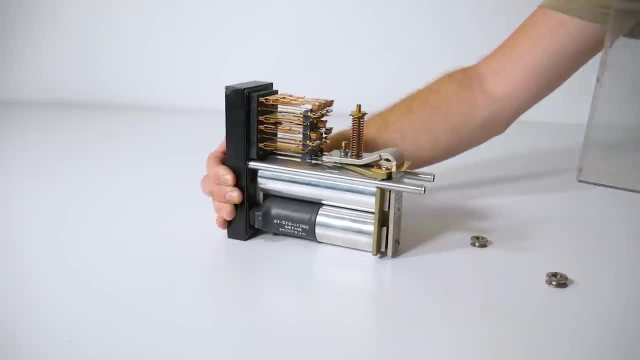 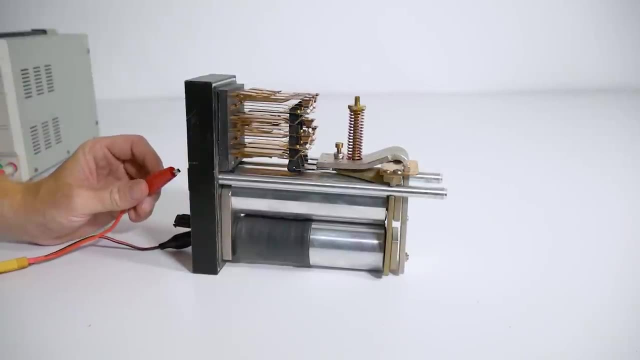 inside and see what it does. I love playing with stuff like this. At its simplest, a relay is just an electromechanical switch, a way to turn something on or off with an electrical signal. When I energize the coil at the bottom, it acts as an electromagnet pulling a lever. 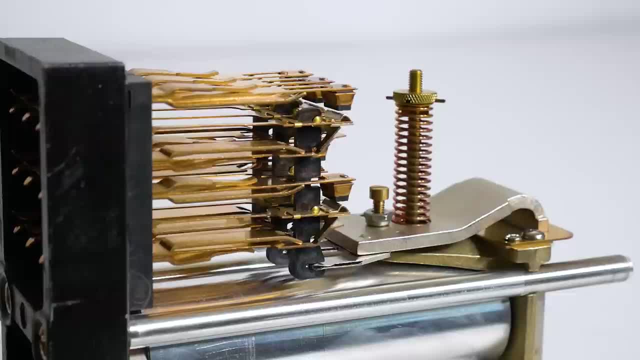 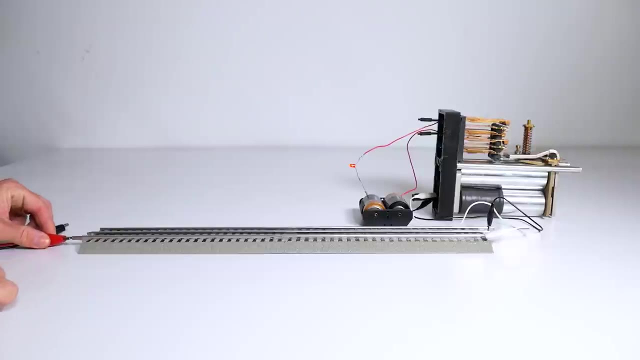 towards it. On the other side of the lever you can see the movement interacting with several electrical contacts. It's a little tough to see here, but these contacts are like switches that can control secondary circuits. Some will be switched on when the relay is energized and others are switched off When the relay is energized or de-energized. 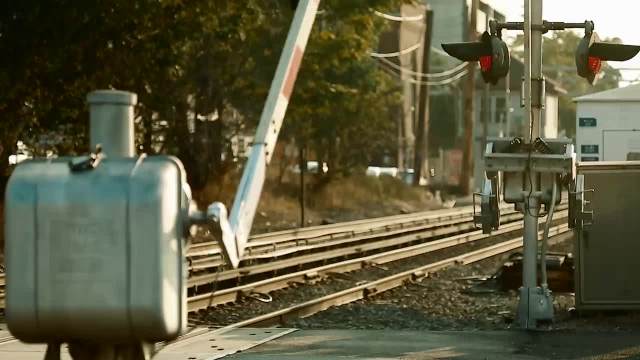 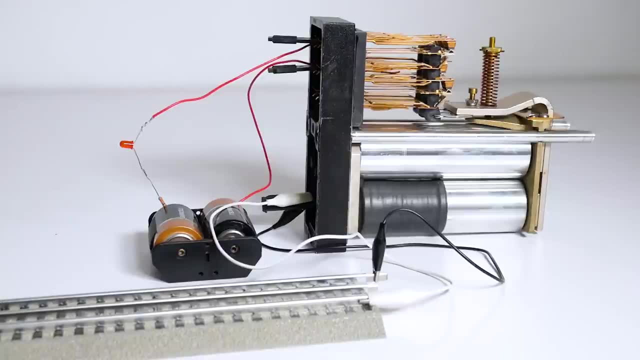 it basically flips the switch on these circuits, allowing various devices like lights, bells and gate arms to be activated or deactivated. In my case, I have a simple battery and LED to indicate whether or not a train is being detected on the rails. When there is no train, 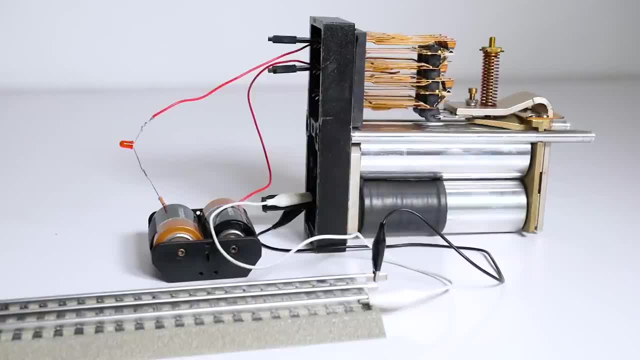 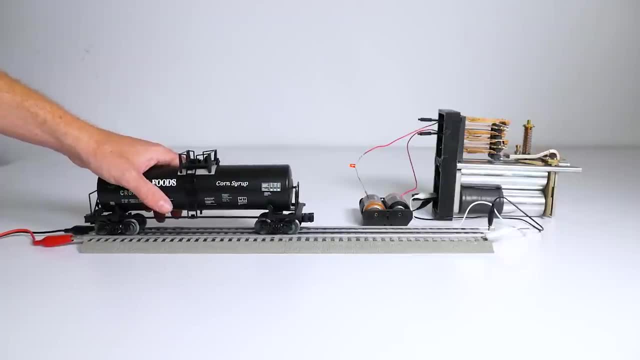 current passes through the relay from one rail to the other, energizing the coil and holding the switch open so the LED stays dark. When I put a railcar on the tracks, the circuit changes. The wheels and axles create a short circuit or shunt a low resistance. 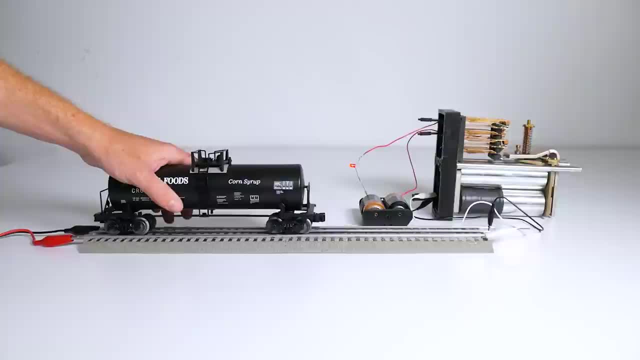 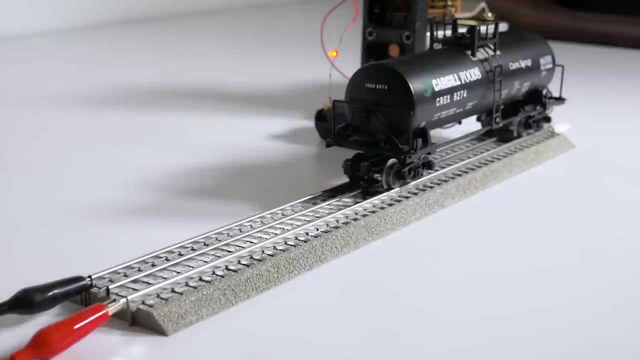 path for the current to flow, essentially bypassing the relay. The coils in the relay de-energize, closing the switch and lighting the LED to warn any nearby tiny drivers that a train is present on the tracks. It all depends on the train giving preferential current path. 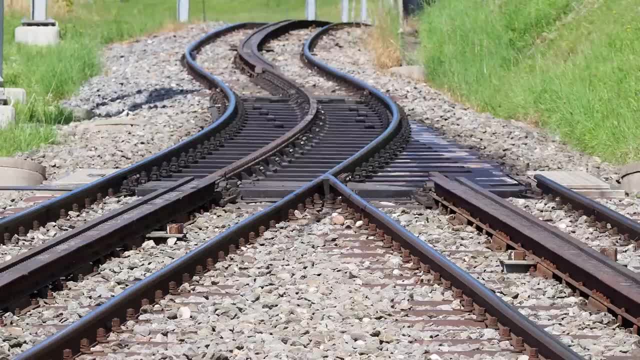 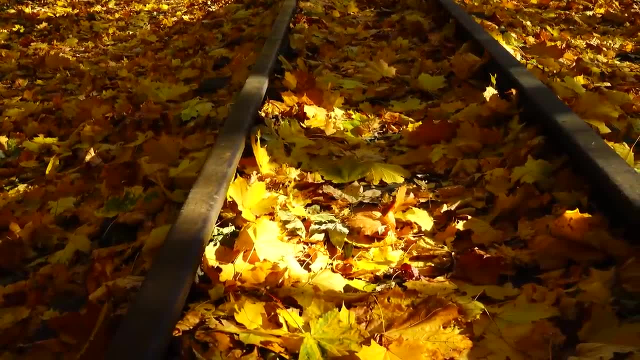 which can be a problem if there are leaves or rust on the rails. You can see how shiny and clean tracks look when they're in frequent use. Tracks that haven't seen a train in a day or more often impose a speed restriction on the first train. 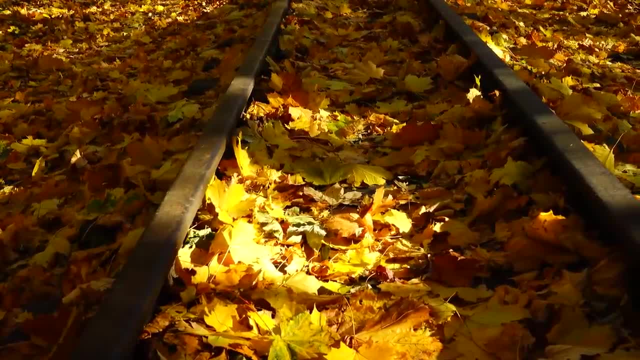 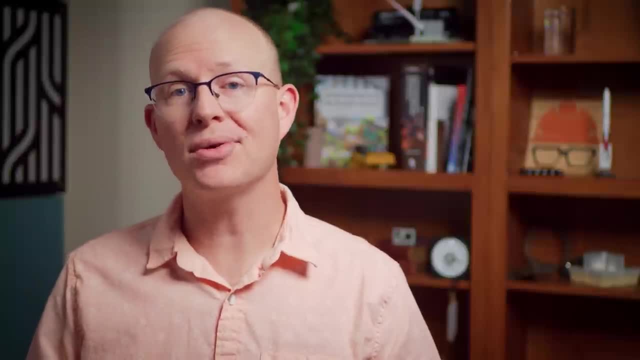 just in case there's rust that could affect the track circuits along the way. If all this circuitry seems a little convoluted to simply detect the presence of a train, it's because of how this simple track circuit handles when things go wrong. 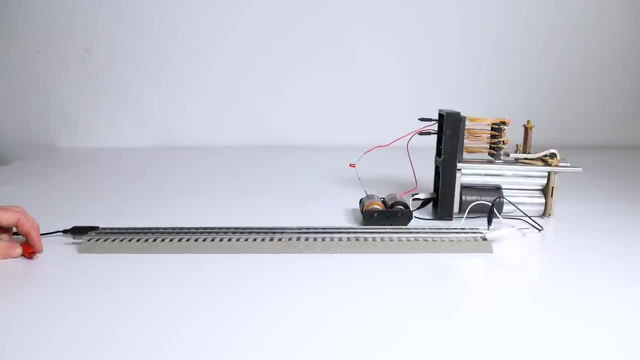 Let's say the track circuit loses power. What happens? The relay de-energizes and falls back to the safest condition, assuming a train is occupying the tracks. Same thing: if a rail cracks or breaks, the relay de-energizes and the light comes on. This is called fail-safe. 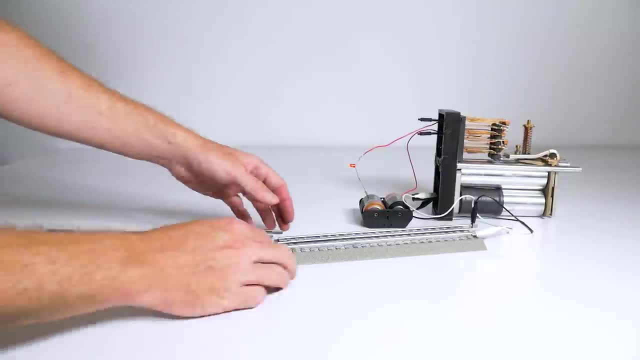 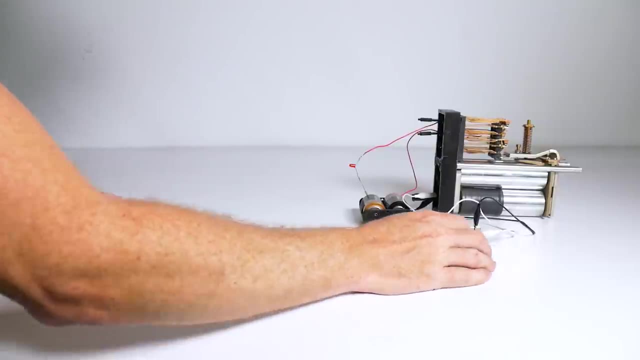 operation or, as the engineers prefer to call it, fail to a known condition. If anything goes wrong, we want the default assumption to be that there's a train coming, because it might be true. Fail-safe operation isn't just in the track circuit, but all the warning. 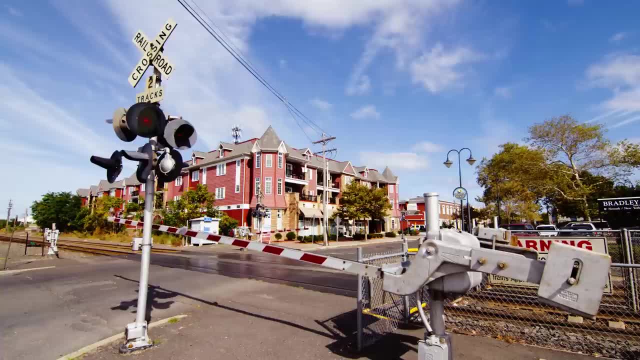 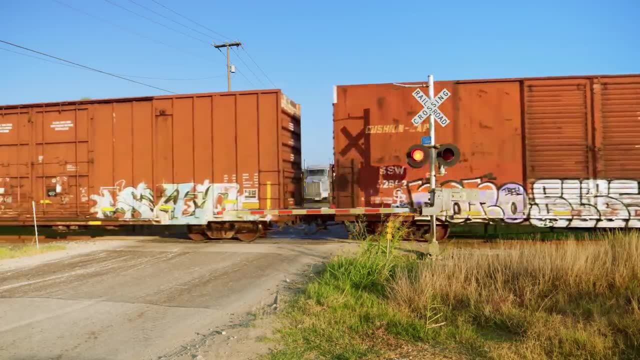 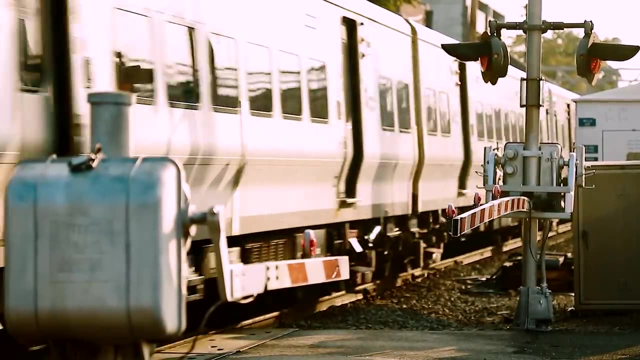 devices too, Like if power's lost. they fall just by gravity alone, And the bells and lights are usually powered by banks of batteries that can last for hours or days. Most modern train detection systems have moved to more sophisticated equipment, but relays are still used around. 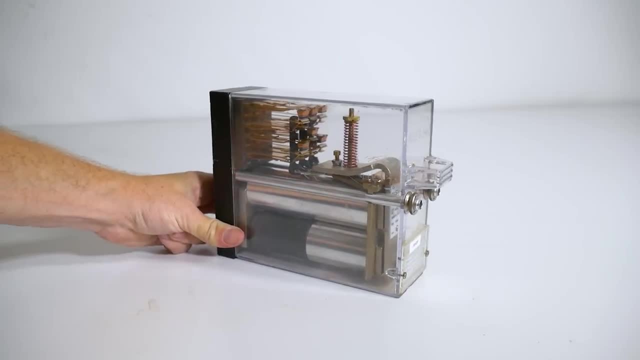 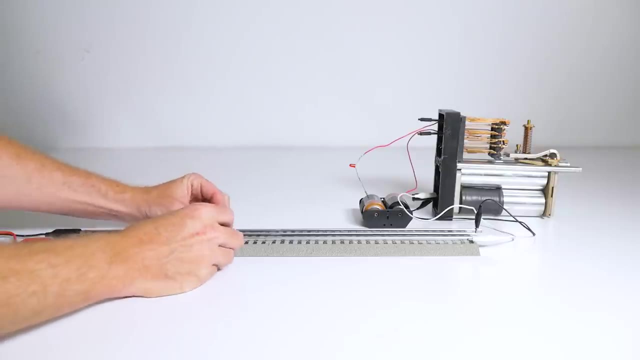 the world because of their reliability. In fact, this is called a vital relay because of all the features that make it extremely unlikely to fail. You can see it acts slowly, so the inevitably noisy signal of a train shunting the tracks can't cycle it on and 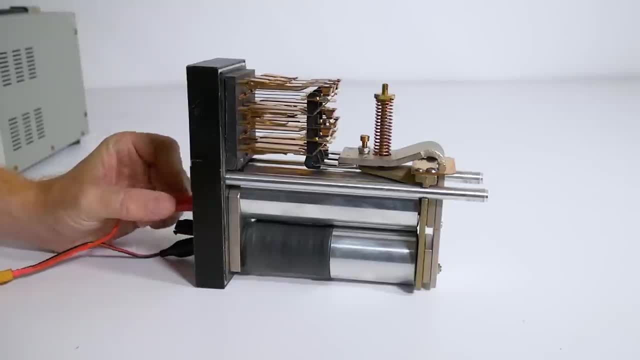 off. over and over, The armature assumes the de-energized position, even if the spring breaks. the contacts use special materials to keep from welding together and they're just really robust and beefy to make sure they last for decades. But even though assuming 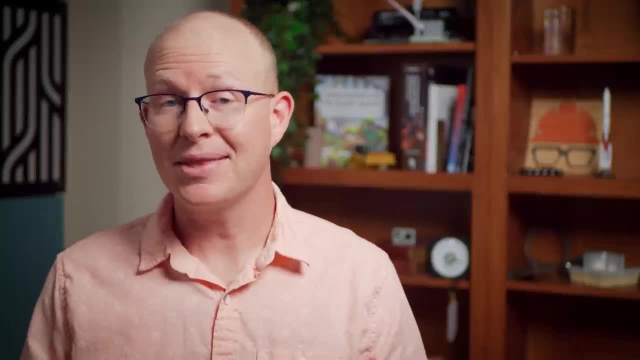 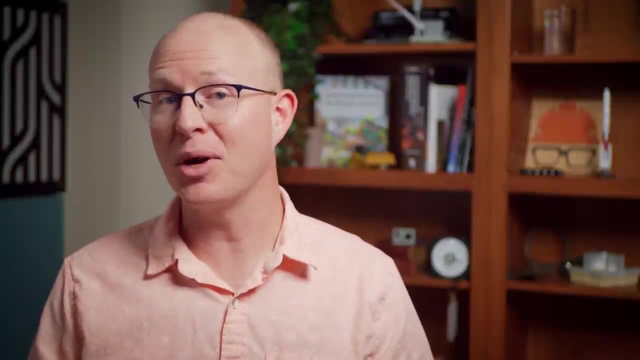 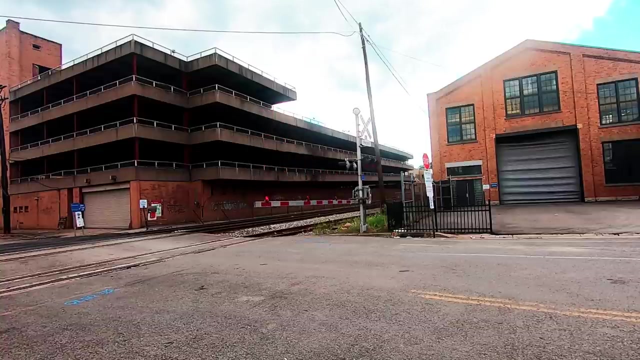 a train is coming is the safest way to manage problems, it's not without its own challenges. Warning devices depend on trust, and that's an extremely tenuous confidence to ask of a motorist. We are naturally dubious of automated equipment. Every time a grade crossing activates and no train comes, that trust is eroded, making 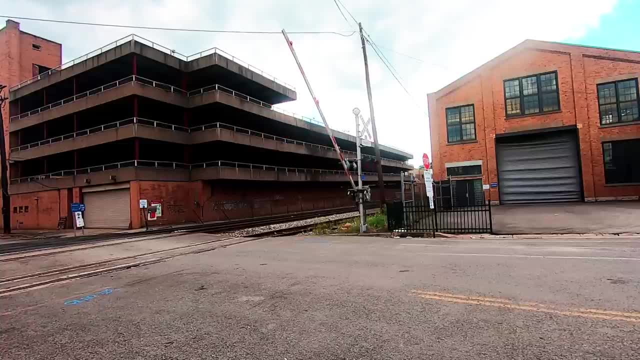 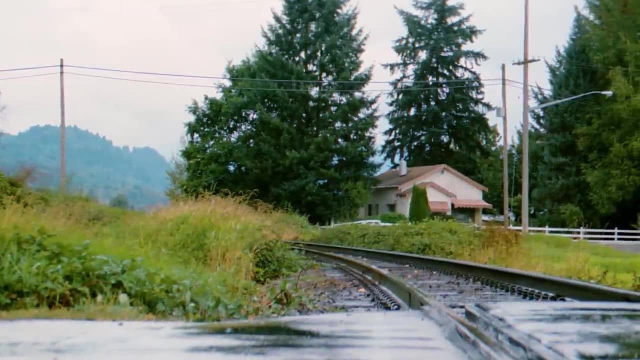 motorists more likely to drive around the gates. So failing safe isn't enough. We also need to make sure the failure is rare. Current leaking between the tracks through water, plant growth or debris can falsely trigger warning devices. so railroads put a lot of time into keeping tracks clean and the coarse. 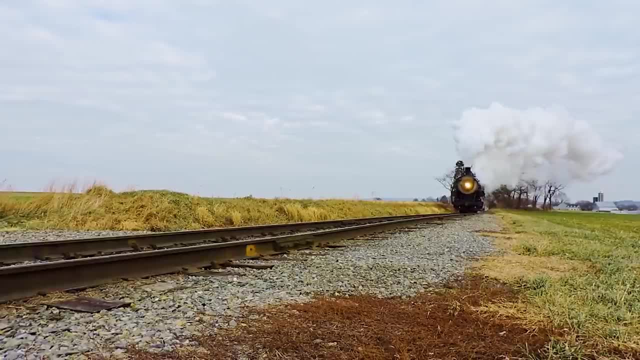 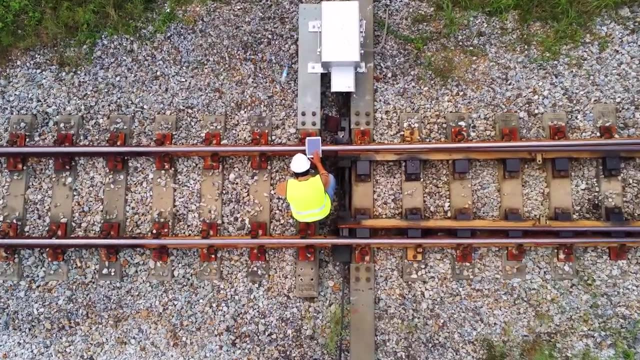 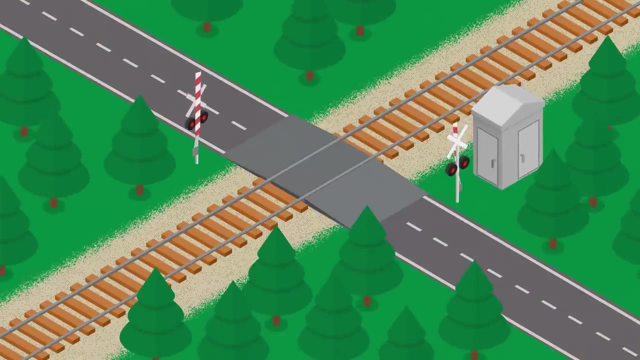 gravel below the tracks, called ballast, freely draining, to prevent water from pooling up. In addition, even though maintenance workers can manually trigger devices by shunting current across the tracks, this is done rarely to avoid impacts to road traffic. But maybe you've spotted a flaw in this simple track circuit. If not, let me point. 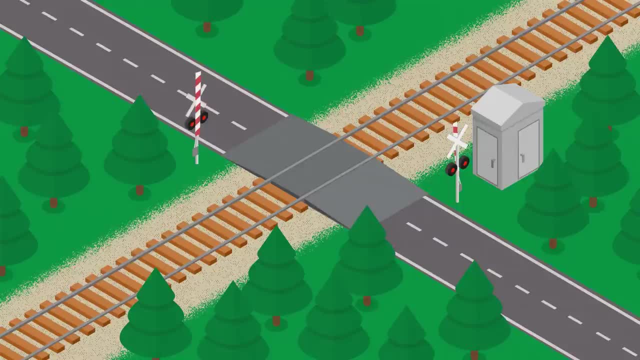 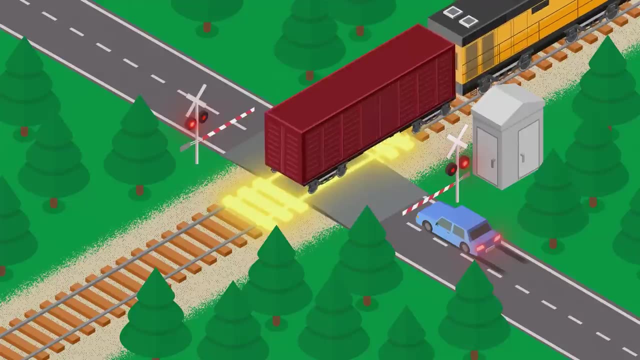 it out. It's all to do with where you put the boundaries. If the circuit is close to the crossing on either side, there's no warning time. By the time the train is detected, the motorist wouldn't be able to clear the intersection or come to a stop. But if the 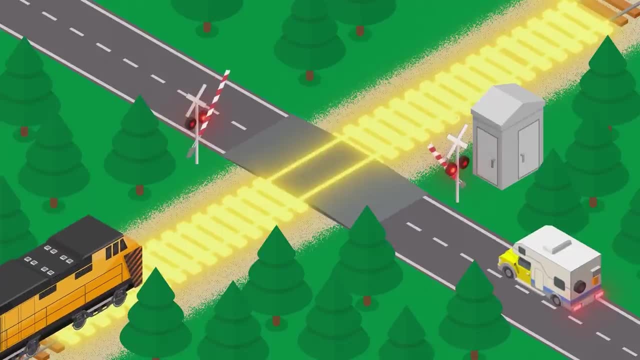 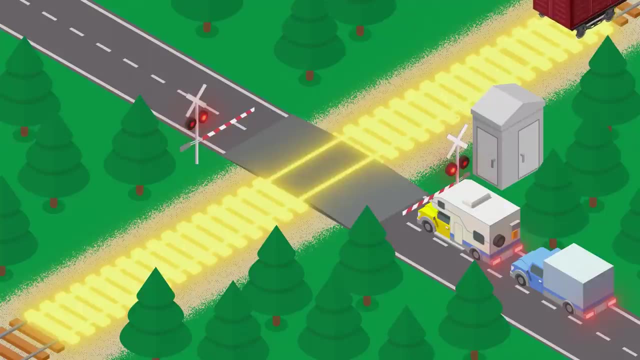 circuit extends far enough beyond the crossing to give adequate warning time, motorists will have to sit and wait well after the train has passed before it comes off the track circuit and the warning devices turn off. So instead of a single track circuit, most crossings use three: Two approaches and an. 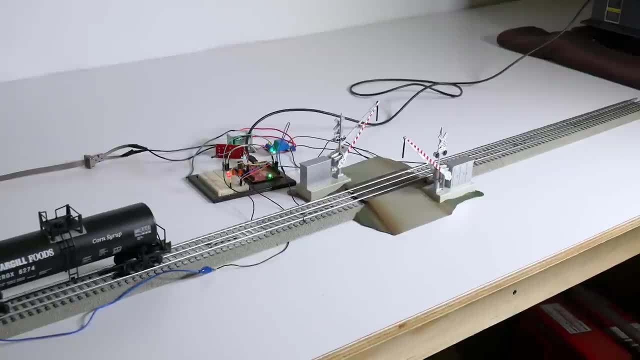 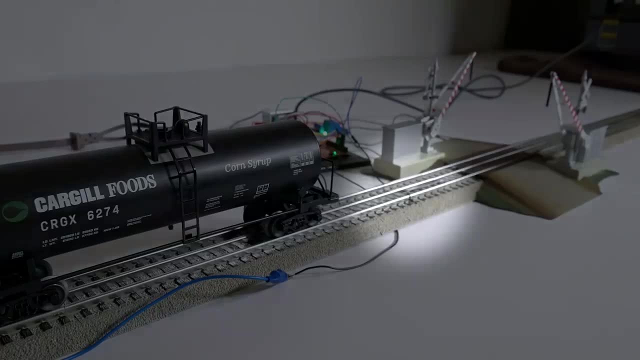 island. Let me show you how this works with another demo. Now I have three track circuits set up, with power going to each one. The rails are separated by a small gap to avoid an inadvertent connection across the circuits On actual railroads. 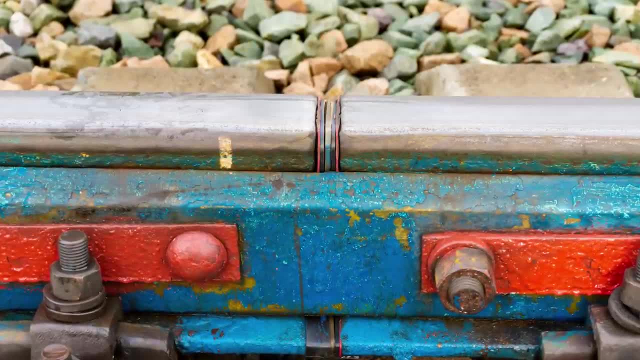 you can often identify insulated joints used to isolate the track from the track circuit. The track circuit can be separated by a small gap to avoid an inadvertent connection across the circuits. On actual railroads, you can often identify insulated joints used to isolate the track circuits. They can be hard to distinguish if the insulating material matches the profile. 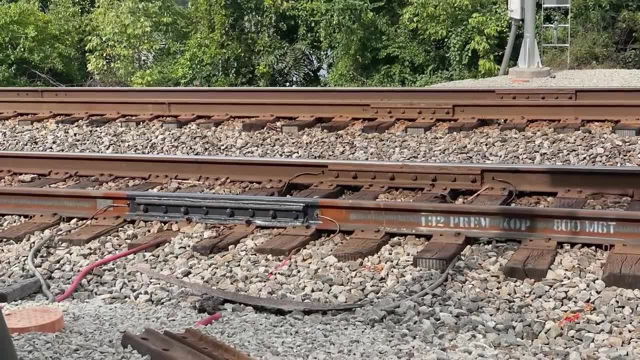 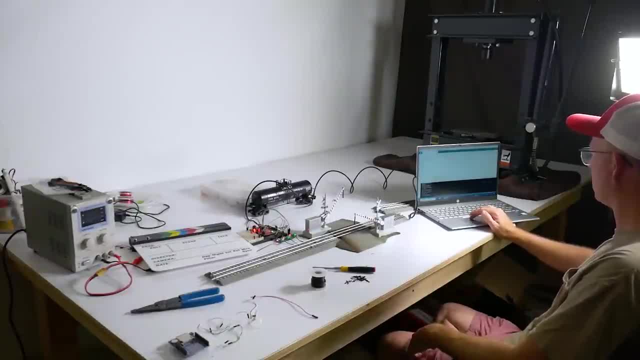 of the rail itself, but they're often painted to be easy to spot. A three circuit configuration requires a little bit of logic to decide when to turn on the warning devices and when to turn them off. So, despite the fact that I have the coding skills of a civil engineer, 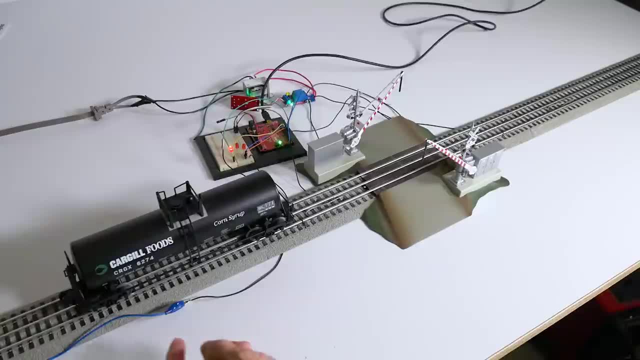 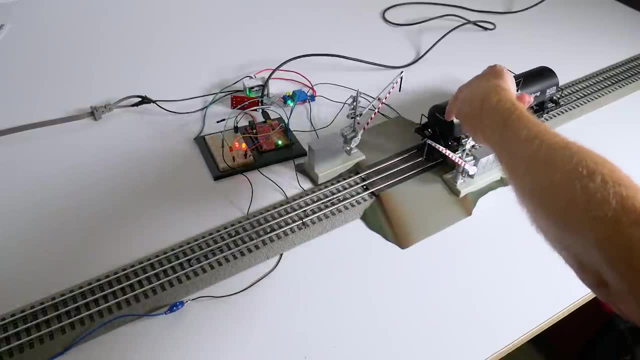 I put this demo together using an Arduino microcontroller. The model railroad. folks are surely shaking their heads at this. You can see my LEDs as I roll the train along the tracks, indicating which of the circuits is detecting the presence of a train From. 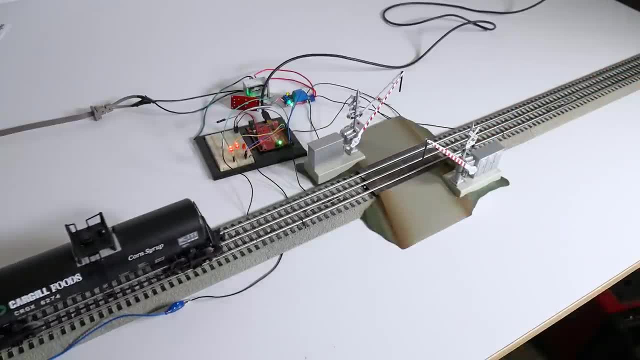 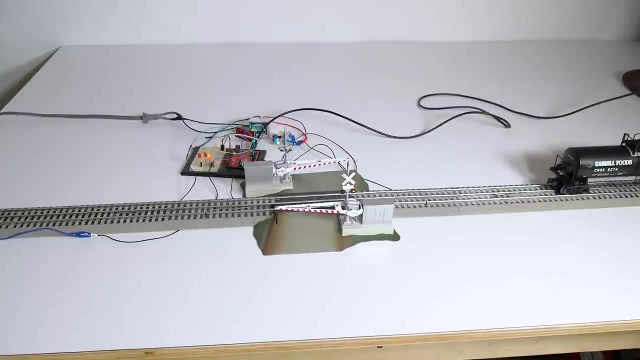 approach to island to other approach. And here's how the logic works: When a train is detected on either approach circuit, it immediately activates the warning devices. The lights flash, bells sound and gates drop As the train keeps moving toward the crossing. 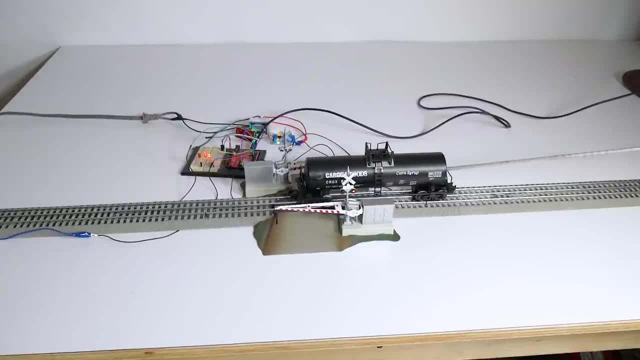 it's detected on the island circuit too. The circuit effectively takes over control of the warning devices. They'll stay on for as long as the train is occupying the island circuit. As soon as the island is unoccupied, the warning devices turn off. Even though one of the approach 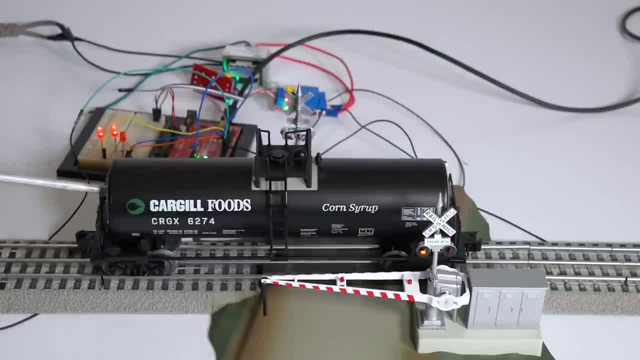 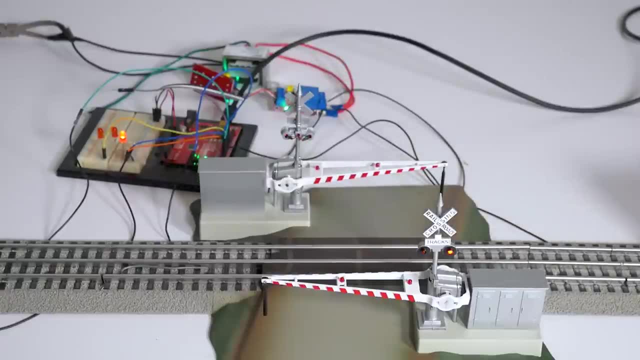 circuits is still detecting a train. You can see how just a little bit of logic makes it possible to give some warning time for motorists before the train arrives at the intersection, without keeping them stuck behind the gates after the train has passed. But how much warning? time is enough. In the US the minimum requirement is 20 seconds between activation of the warning devices and the arrival of a train, but it's typical to see 30 or 45 seconds. You might think the more warning time the better, but it's a balance. Too much warning. 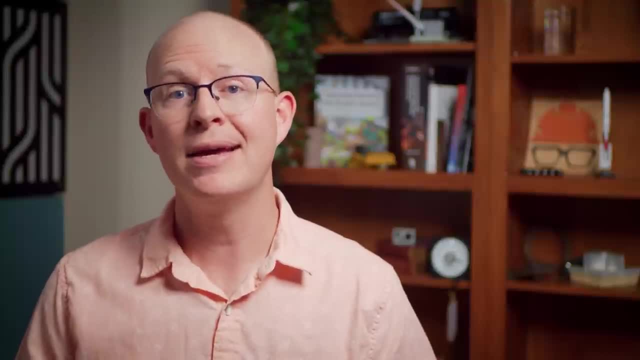 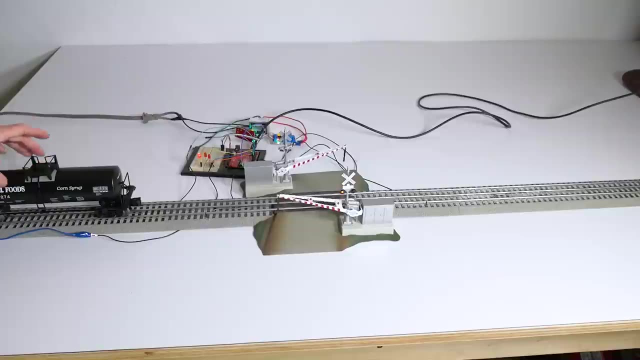 time and motorists might become impatient and drive around the gates. so more time can actually make crossings less safe. For the three-circuit example in the demonstration, the only control you have over warning time is where to start the approach circuit, The farther away from the crossing it begins. 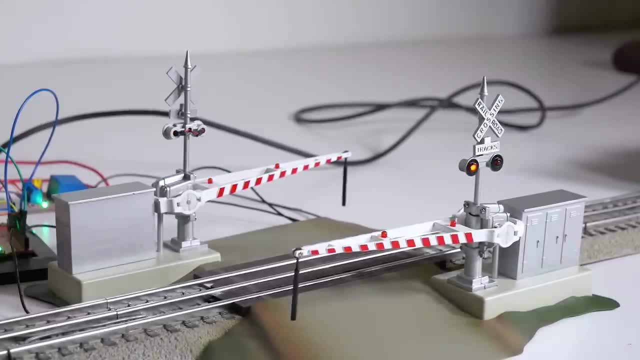 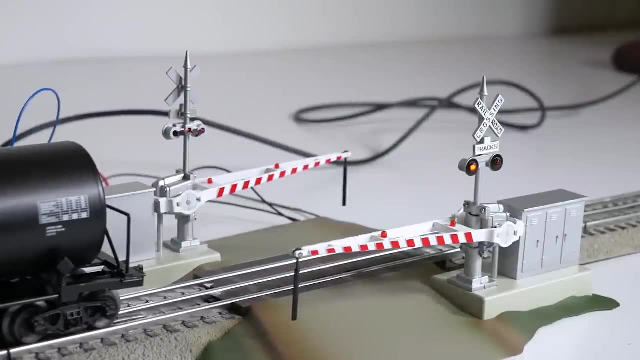 the more warning time you get, But the exact time depends on the speed of a train, Since the approach is fixed in place. a slow train will provide lots of warning time- This is more current warning time- and a fast train will provide less And a train stopped on. 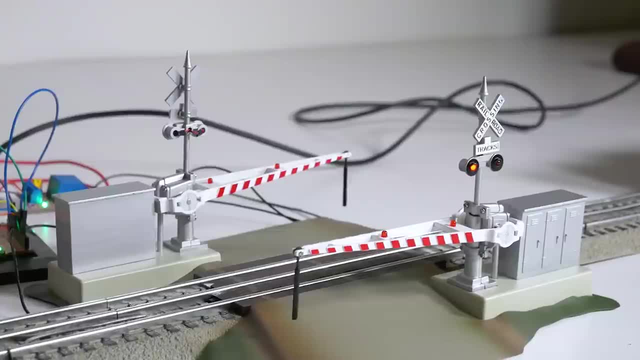 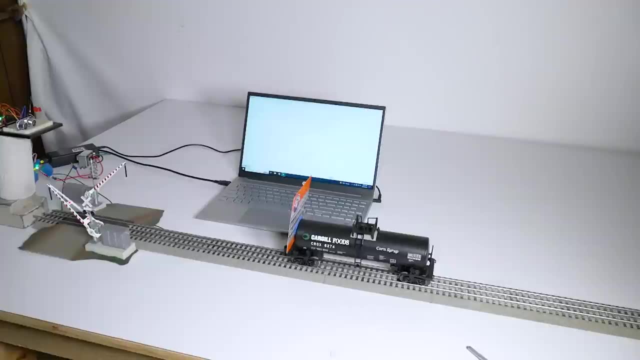 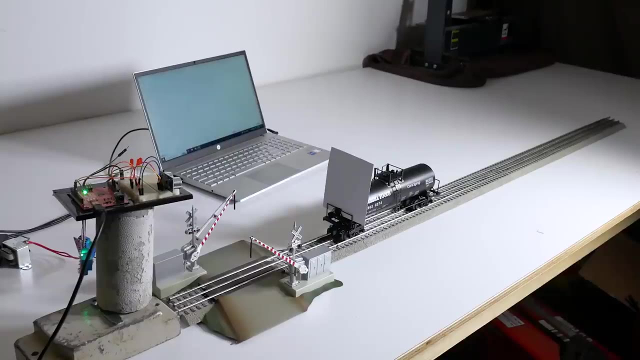 an approach circuit before it even reaches the crossing will hold the gates down indefinitely. So the next step in grade crossing complexity takes speed into account. I put a little acoustic distance sensor on my Arduino so that I can try to estimate the speed of an oncoming train. The large cardstock cutout just helps my sensor see the train. 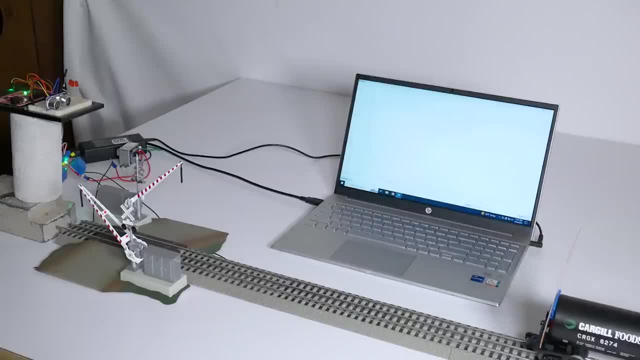 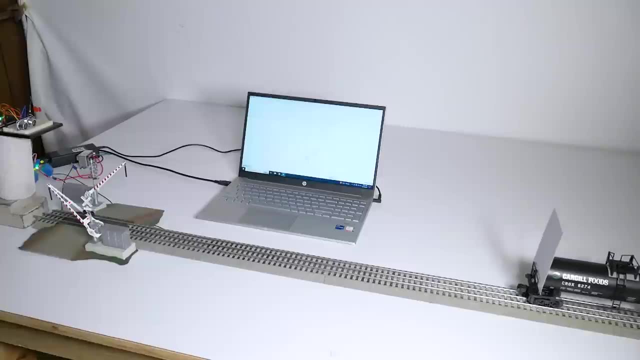 a little better. The Arduino measures the distance over time, converts that to an approximate speed. it will take the train to arrive at the crossing. If the expected arrival time is longer than the warning time I programmed in, nothing happens. But if an arrival is expected within, 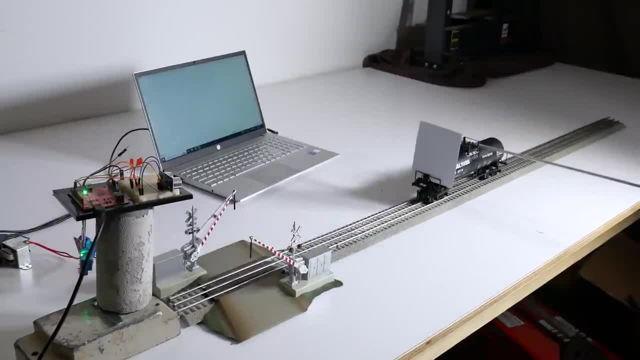 the warning time the devices are activated. You can see: if I approach the intersection slowly, the gates don't drop until I'm relatively close to the crossing, And if I speed things up, the gates drop when I'm farther away, anticipating the faster arrival. 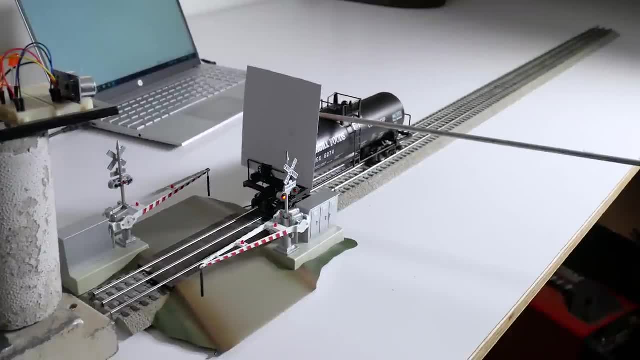 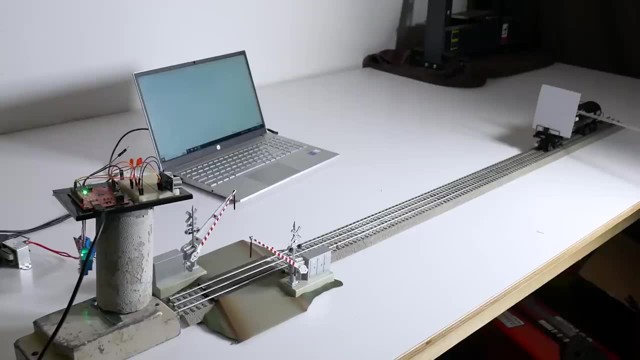 of the train. In theory, this type of sophistication means that the warning time at a crossing will always be the same, no matter the speed of the train. But it doesn't just solve that problem. If you've ever sat at a railroad crossing while a train has stopped on the 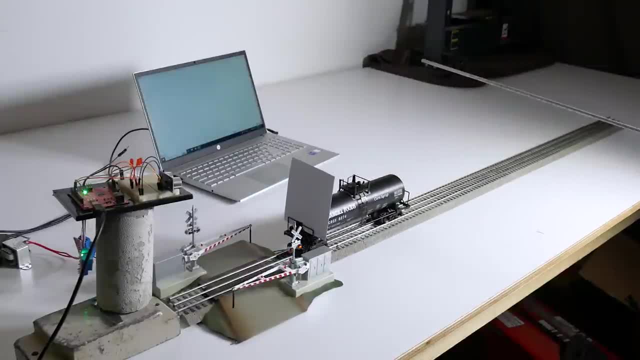 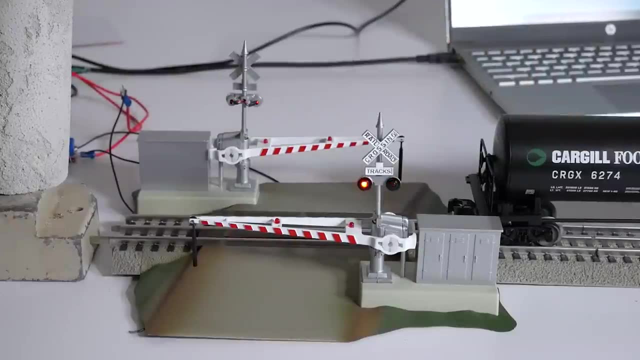 approach circuit. you know the frustration it causes. A grade crossing predictor avoids the issue. You can see as I move my train toward the crossing: the devices activate, assuming the train will cross, But when I stop short, the predicted arrival time goes effectively to an error. 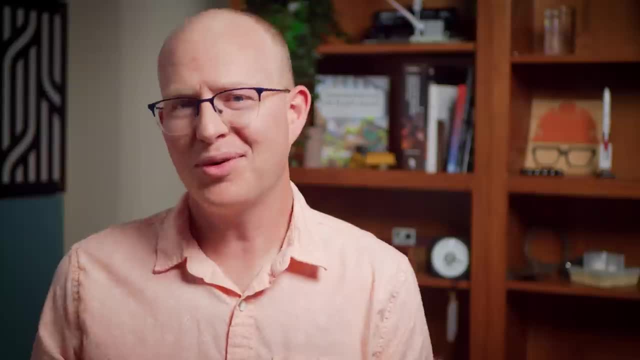 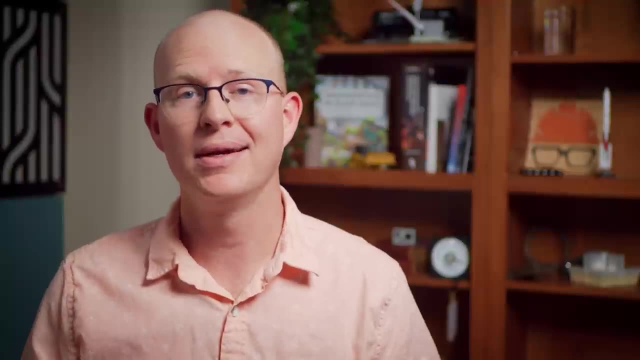 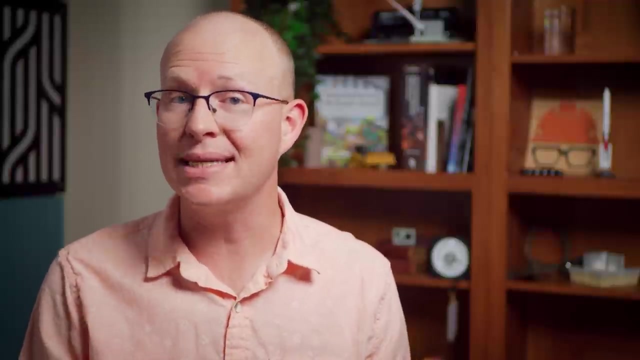 Of course, actual crossings don't use sonar to predict the speed of a train. In most cases, they use track circuits with an alternating current. A train interacts with the frequencies of the circuit as it travels along the rails, giving the sensors enough information to detect. 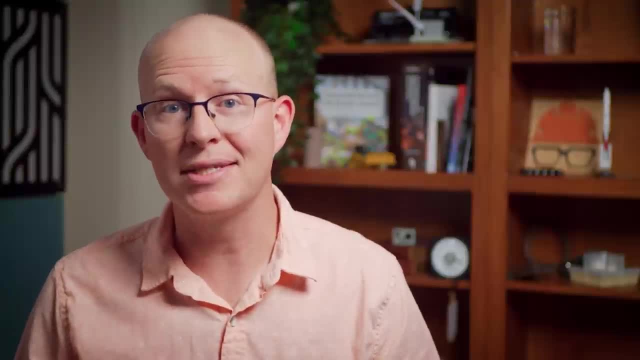 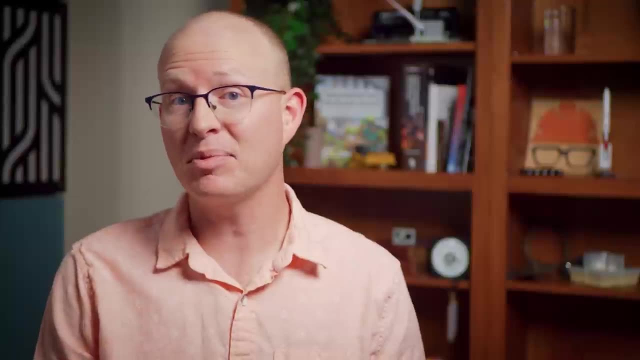 the presence and speed. Sometimes you can even hear these frequencies, since they're often in the audible range. AC track circuits are also used for electric train systems because they're less susceptible to interference from the traction of the train. So if I'm in the audible range, I don't have to worry too much about the train. 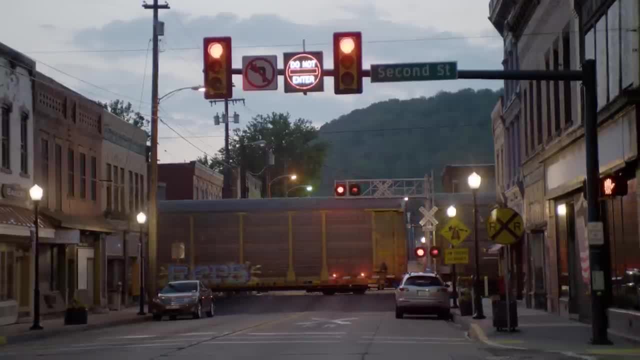 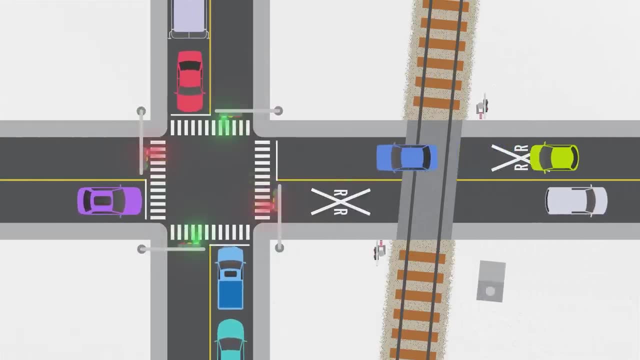 Another challenge with grade crossings happens in urban areas where signalized intersections are present. near the railway, Red lights form a line of vehicles that can back up across the tracks. You should never drive over a railway until you know it's clear on the other side. but if you're not paying attention it can be easy to misjudge the available space. 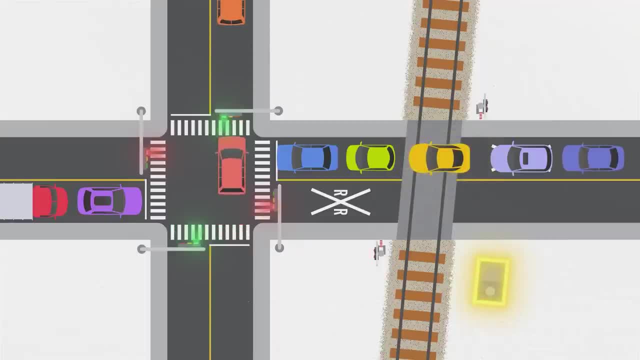 and find yourself inadvertently stopped right on top of the tracks. Traffic signals near grade crossings are usually used to predict the speed of the train, But if you're in the audible range, they're usually coordinated with automatic warning devices. When a train is approaching, the signal goes green to clear the queue blocking the tracks. Equipment for 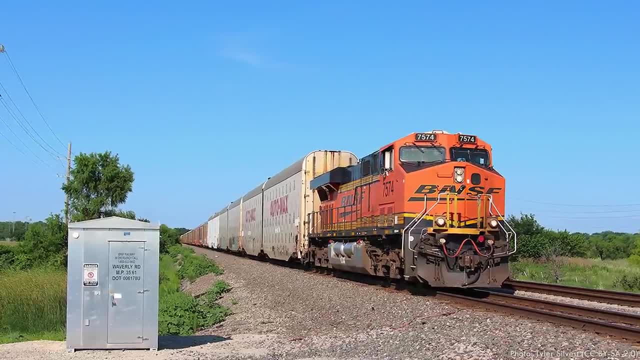 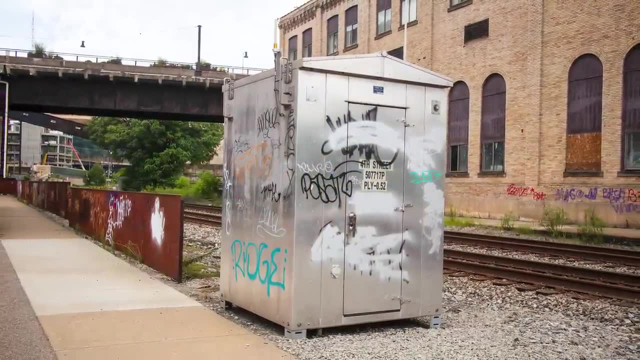 the most basic track circuits to the most sophisticated, including relays, microcontrollers, backup batteries and more, are usually housed in a nearby bungalow or cabin that's easy to spot. In the US, every grade crossing has its own unique identifier, and they all have. 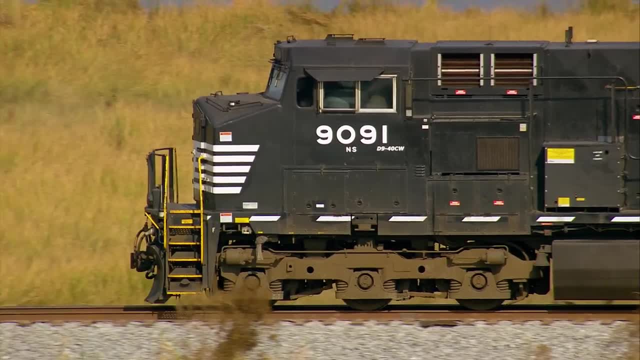 a phone number to call if something isn't working correctly. Railroads take reports seriously, so give them a call. If you're in the audible range, you'll be able to call if you ever see something that doesn't look right. If you want to see a lot of these, 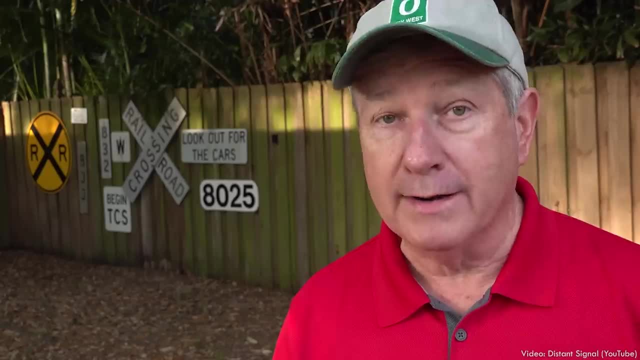 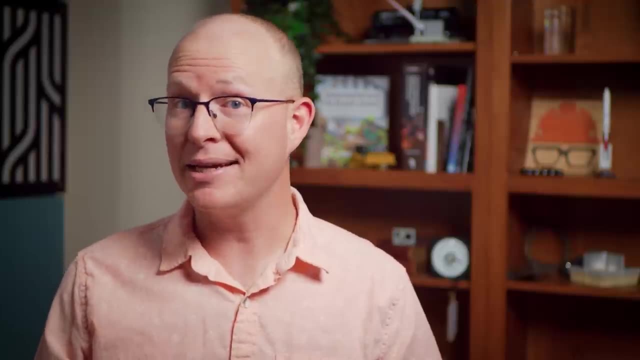 grade crossing systems in action. check out my friend Danny's channel, Distant Signal, for some of the best railfan videos out there. We depend on trains for a lot of things and, in the opinion of many, we could use a few more of them in our lives, Despite the hazard. 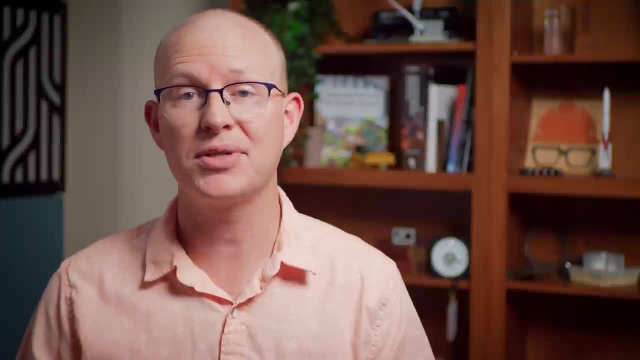 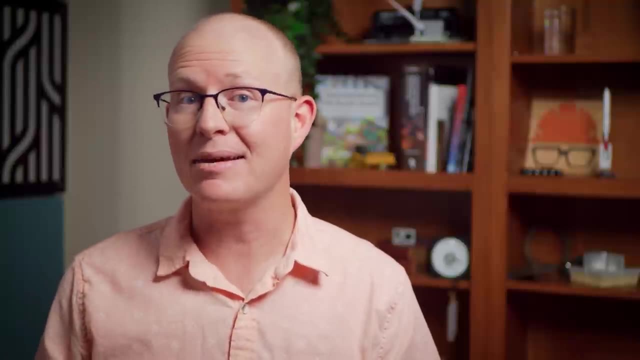 they pose. trains have to coexist with our other forms of transportation. Next time you pull up to a crossbuck, take a moment to appreciate the sometimes simple, sometimes high tech, but always quite reliable ways that grade crossings keep us safe. 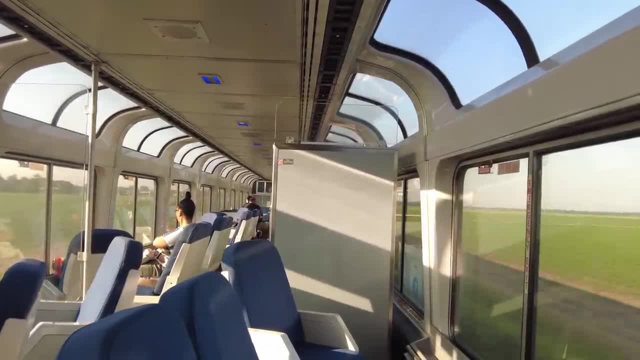 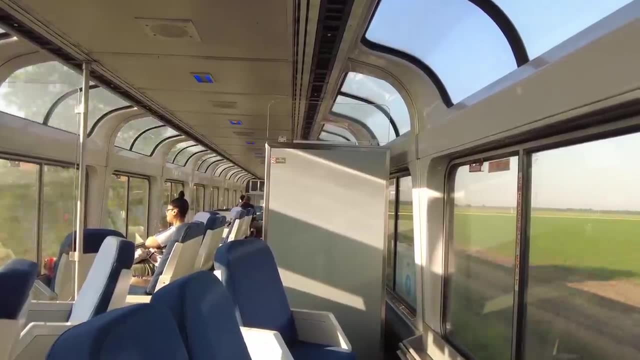 I've talked about what it's like as a motorist at a grade crossing, but I didn't mention how satisfying it is to be a train passenger, watching those lines of cars wait as you pass by. Where I live, I don't get to take many train rides, to the dismay of 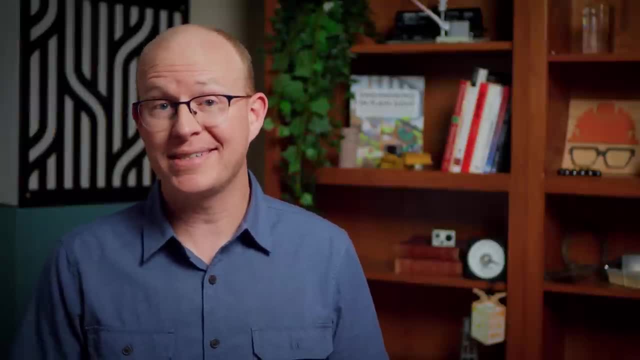 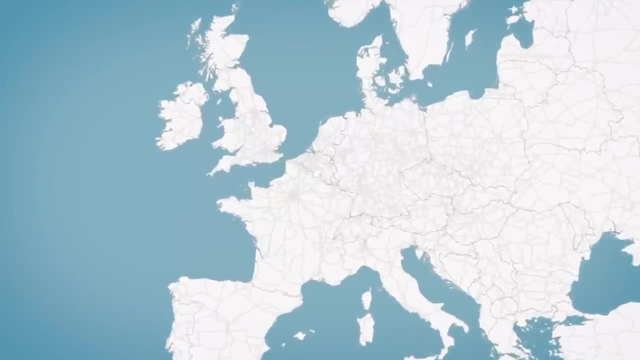 my obsessed three-year-old, but I do have a show that scratches the itch. Jetlag is a travel-based game show created by my friend Sam of Wendover Productions. Each season is a year to complete challenges using different modes of transportation. It's just such. 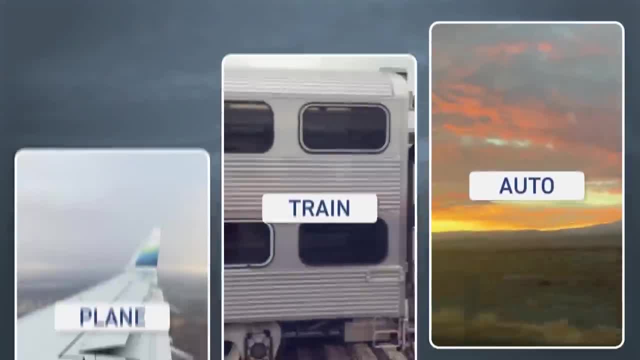 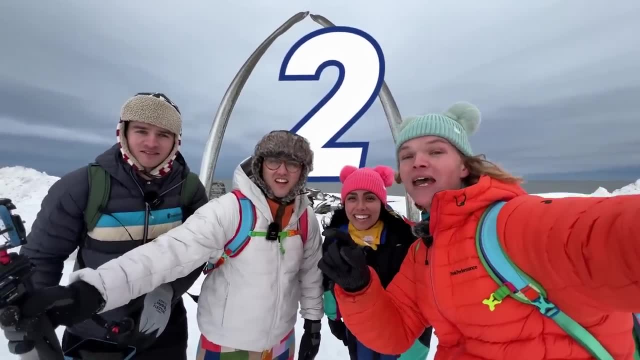 a creative idea, and what I really love is seeing how all types of public transport function around the world. Season 8 is in full swing right now. You can watch a few episodes on YouTube, but if you want to catch each one as it's released, you have to do it on Nebula. 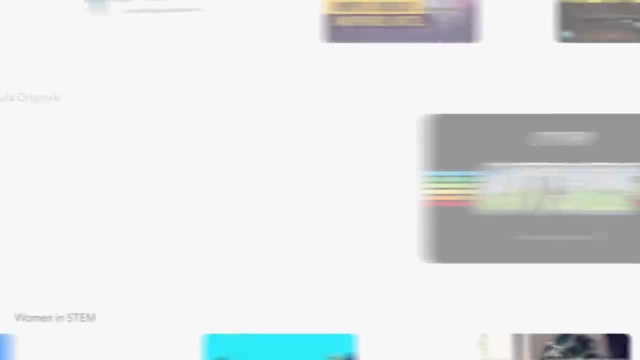 You've heard me talk about Nebula before. it's a streaming platform for independent creators. like me, I love YouTube and it's a perfect home for most of the videos I like to make, but the platform does strive to keep me up to date with the latest news and updates. 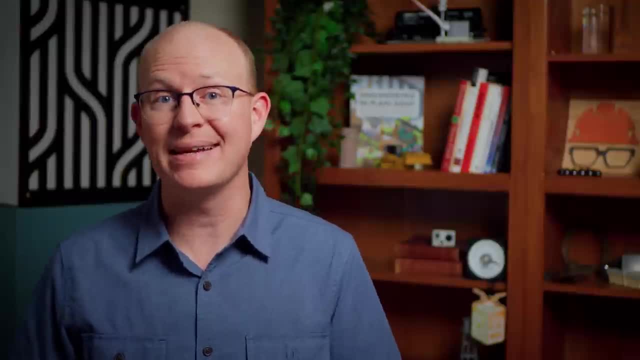 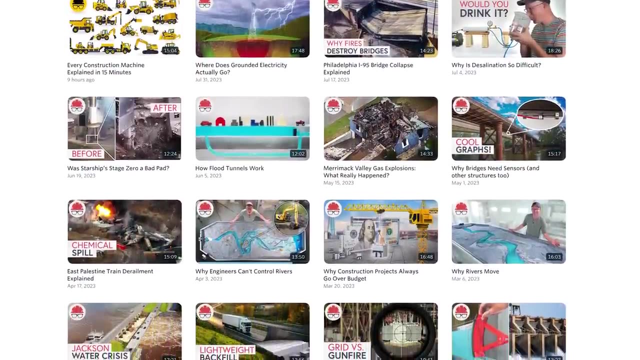 I'm Sam of Wendover Productions and I'll see you next time. the types of content that succeed Series don't work very well. every video has to be optimized for clickability and everything is ad-supported, which constrains not only the content of the 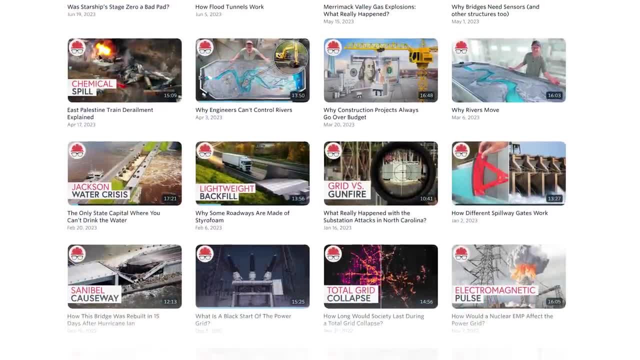 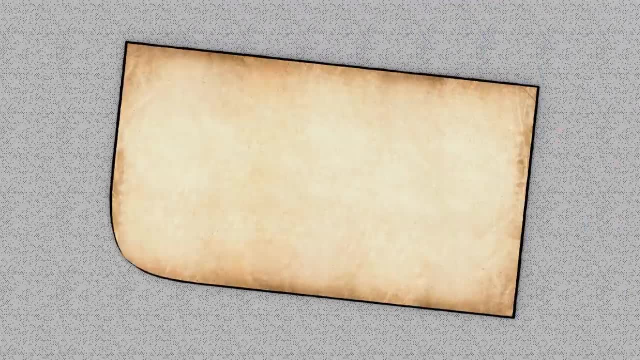 videos, but also how much room there is for experimentation. Just like everything on TV eventually turns into a reality show, it seems like everything on my part of YouTube eventually becomes a 15-minute explainer with flashy graphics and a clickbait thumbnail. Don't get me wrong. 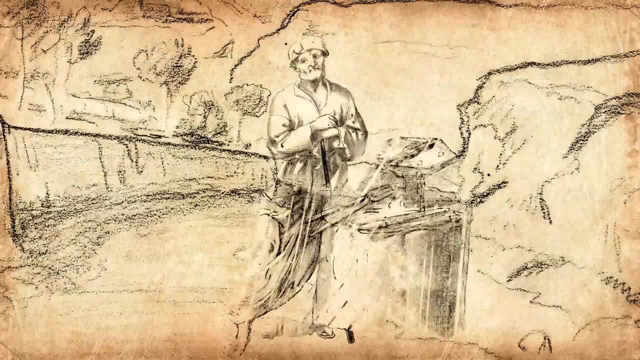 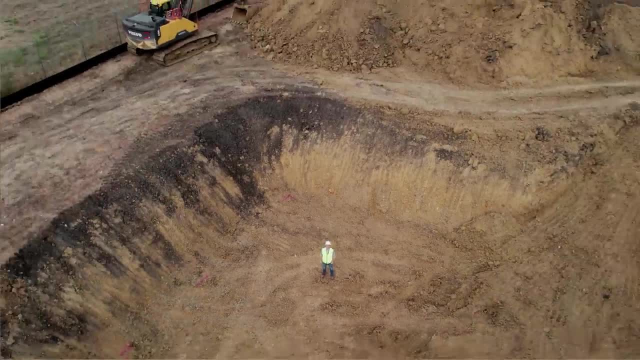 I love a good explainer with flashy graphics, but I like other stuff too. Shows like Jetlag and my Practical Construction series, where I embedded with a contractor for a year while they built a sewage lift station, don't fit that YouTube mold, but they're also too weird. 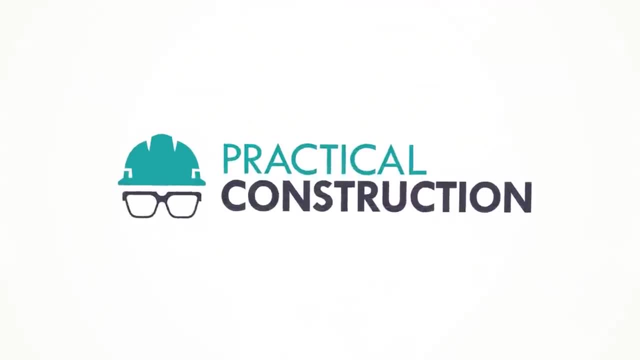 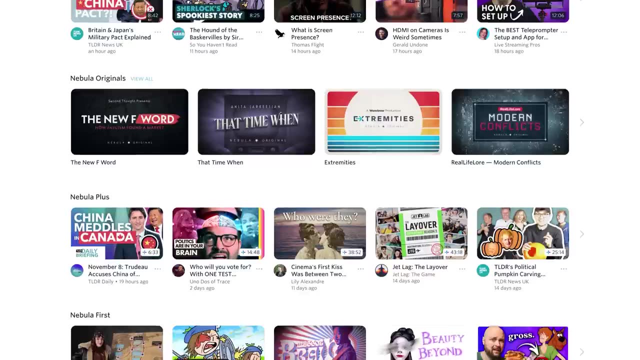 for a big studio to greenlight Nebula meets us in the middle. The platform has grown so much since I started releasing videos there, with tons of exclusive content and early access to your favorite creators' videos, all with zero ads. I know there are a bunch of streaming services. 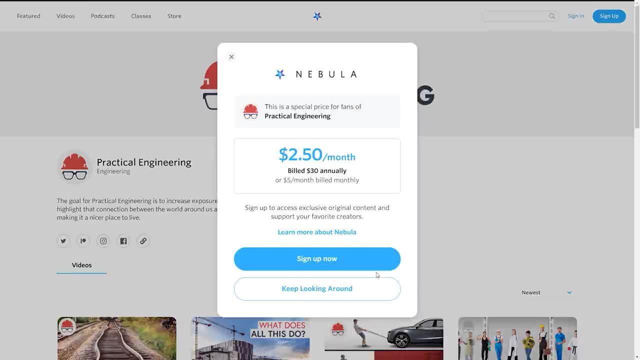 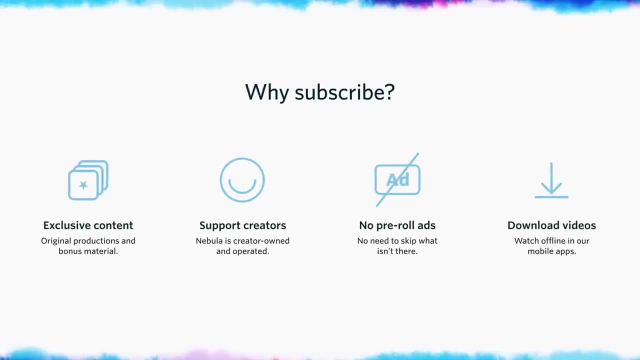 right now and adding another one to your list is a big ask, but at only $30 for an entire year of access, if you use my link, this one's not going to break the bank At that price. it's easy to give it a shot and see if you like it as much as I do That link. 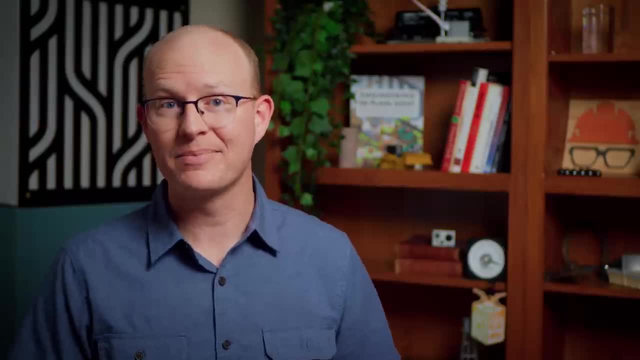 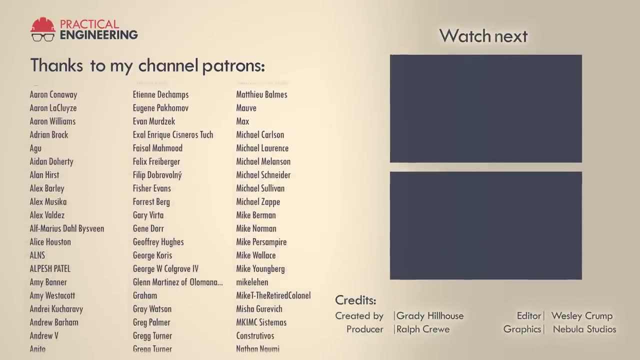 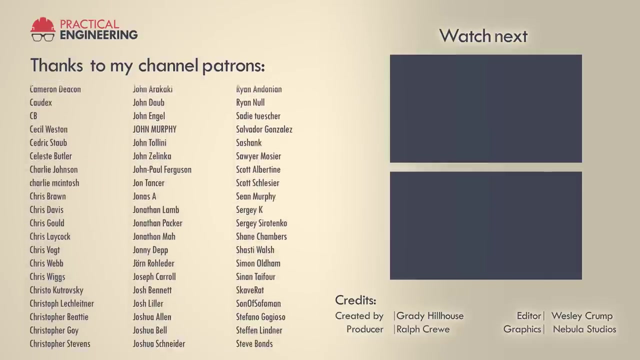 is in the description. Thank you for watching and let me know what you think. Subtitles by the Amaraorg community.